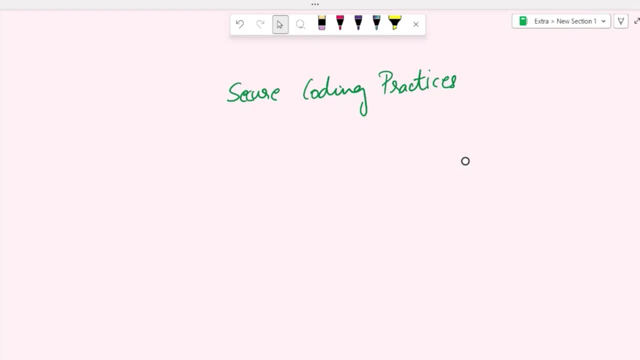 Hey guys, welcome to Cyber Platter. Today we'll learn about secure coding practices. okay, So what are secure coding practices? It is a set of rules or guidelines, techniques or, you know, best practices that are used by the developers when they write a code, software code. This is 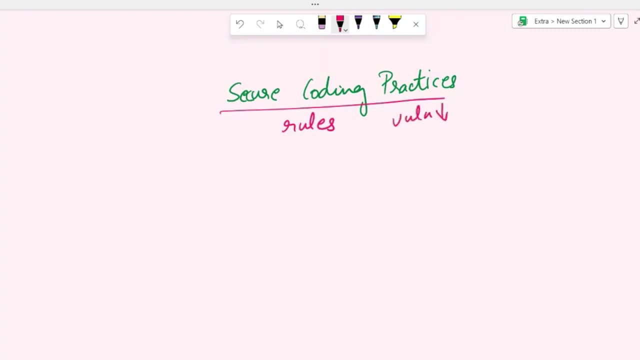 mainly to minimize the security vulnerabilities and mitigate the potential risks. You need to follow secure coding practices to prevent unauthorized access, any data breaches and various types of attacks on software applications. Now let's discuss some of the key secure coding practices. The first coding practice that we'll discuss is input validation. This is a process. 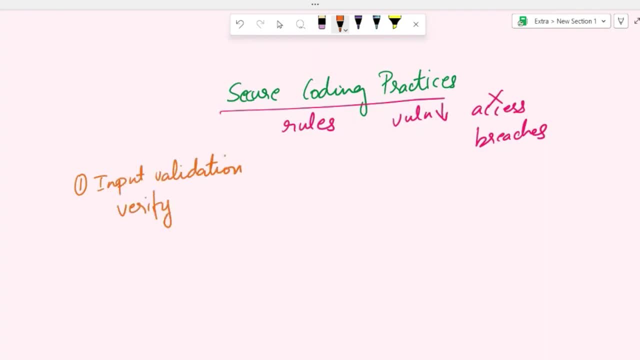 to check and verify the information or data that a user enters into a software application. okay, It makes sure that the data is safe, it is valid and it is in some expected format. okay, Think of it like a gatekeeper. you know who's. 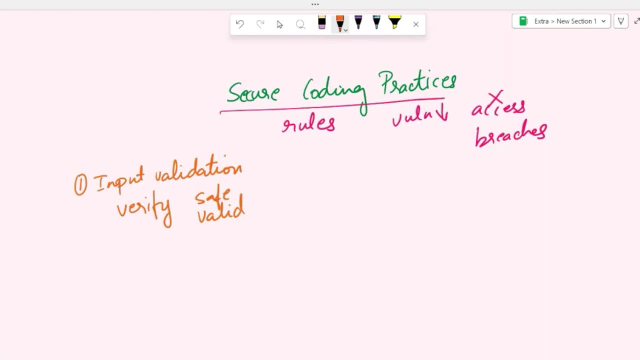 checking who's entering a party. okay, Gatekeeper's role is to make sure that only invited guests get inside the party, right? Exactly like that in software. input validation acts as a gatekeeper to filter out any harmful or incorrect information. Let's look at some of 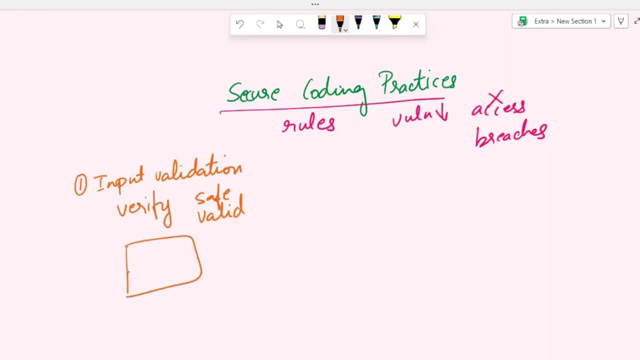 the examples of input validation. Suppose say, there is a form on a portal website that you need to enter your age. So here you can make sure that only numbers are allowed for any user to input the data, because it is age, and you can also make sure that the age is between a. 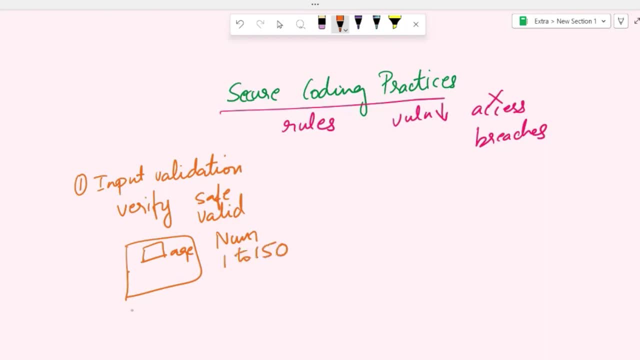 reasonable range, like, for example, say, 1 to 150.. Another example is email validation. Suppose say you're signing up for an account. input validation ensures that the email address entered follows the correct format. like you know, at gmailcom, right When you're creating a password, you can. 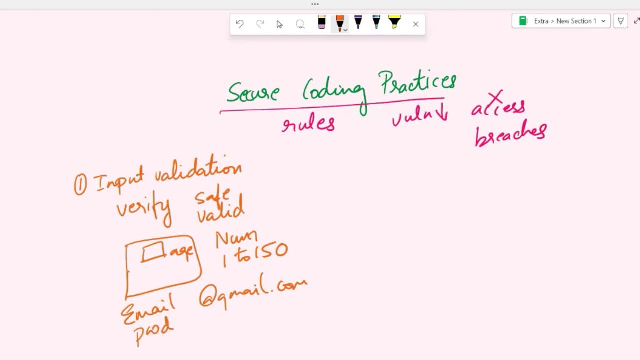 input validation is used to check the password strength. Input validation needs certain criteria, like you know: minimum length, inclusion of both letters and numbers. there is one special character: Even when you upload files, it can check for the size. only so-and-so size is allowed or this file type is allowed. you know this can help to prevent. 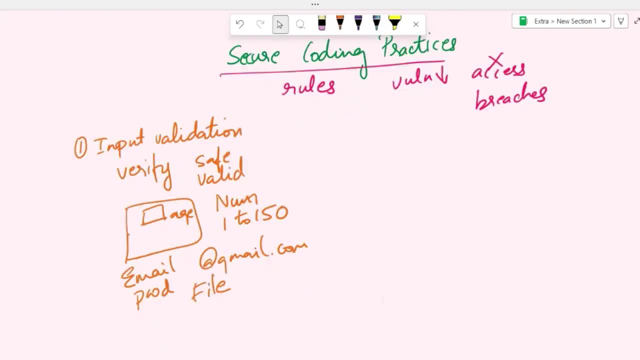 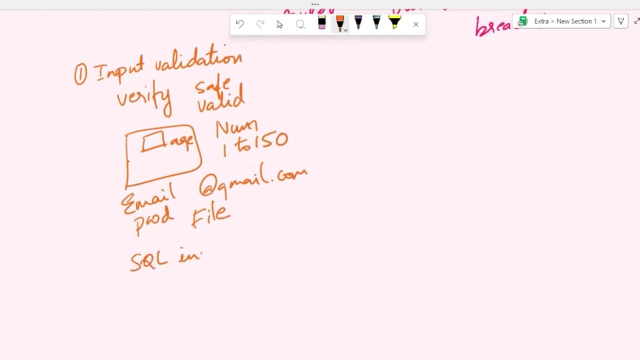 uploading any potentially harmful files. okay. Input validation helps to protect the software application from various types of attacks. okay, Like, for example, if you have a file that is encrypted, for example, SQL injection, cross-site scripting. it prevents data corruption by 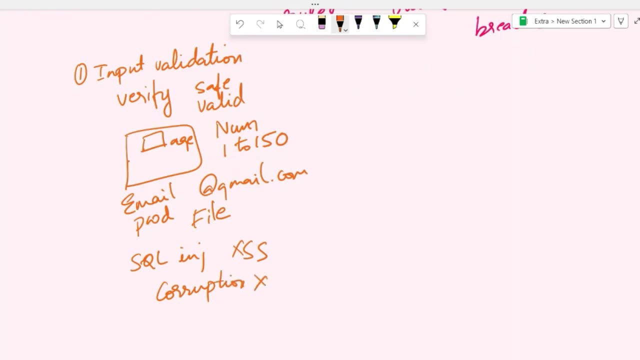 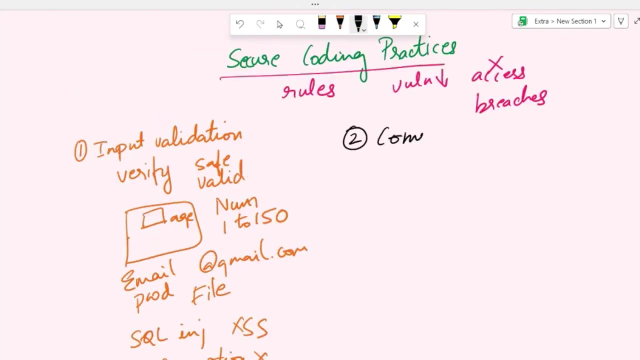 ensuring that only valid and expected data is accepted. It helps maintain the integrity of the application's data. Another coding practice that we'll discuss is secure communication, That is, it is a practice of employing encryption and secure protocols to protect data that is transmitted over networks. okay, This makes sure that the data is confident. 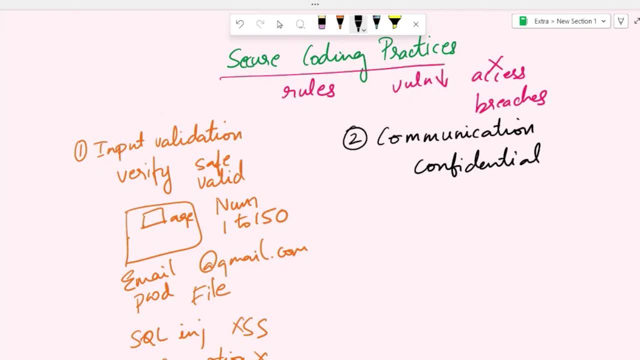 confidential and that cannot be easily intercepted or tampered by an unauthorized individual. Like, for example, you are encrypting your data and then you are using secure protocols like, for example, HTTPS, SSL, TLS, to provide a secure channel for data transmission between a client. 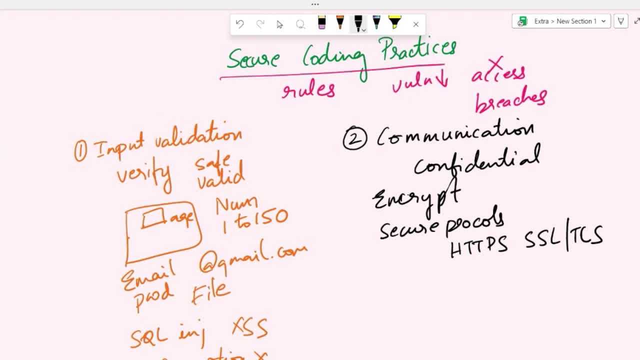 like, for example, a web browser and a server. So these protocols establish an encrypted connection- okay- between the client and the server and make sure that, make sure that the data exchange between them remains confidential and protected, and then we can use authentication, authentication steps, make sure that the client and the server- right, they know each other. this 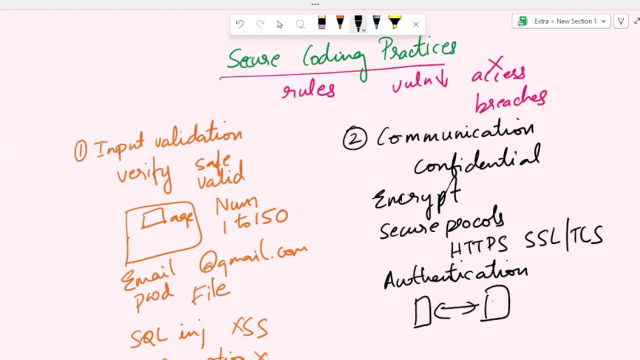 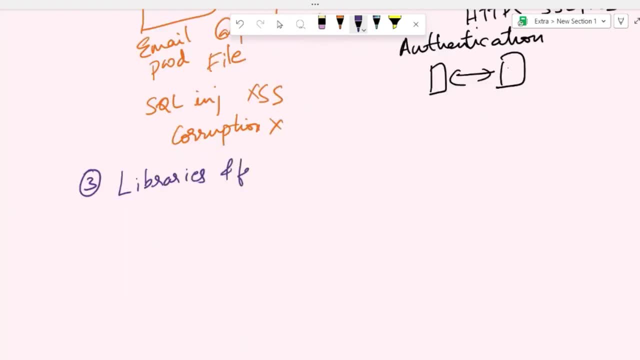 is to prevent any unauthorized entities from intercepting or impersonating the communication. okay then the third practice is use of secure libraries and frameworks. so we have to make sure that only well-known and reputable libraries and frameworks that have like a great track record of being secure and regularly updated are being used in your applications, like, for example, instead. 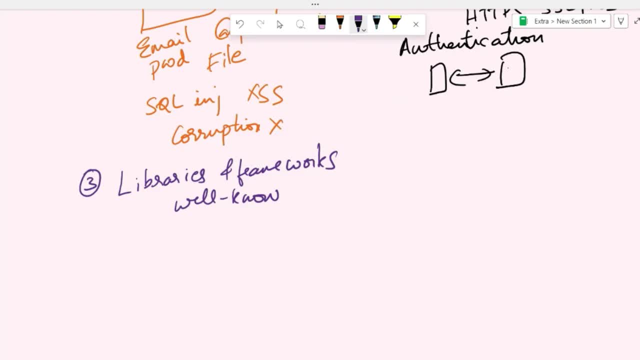 of writing your own encryption algorithm, you can use well-known library like open ssl or bcrypt. or, instead of creating your own password management system, you can use a well-known and tested library to manage your passwords. and then we have authentication and authorization. authentication: make sure to verify the identity. 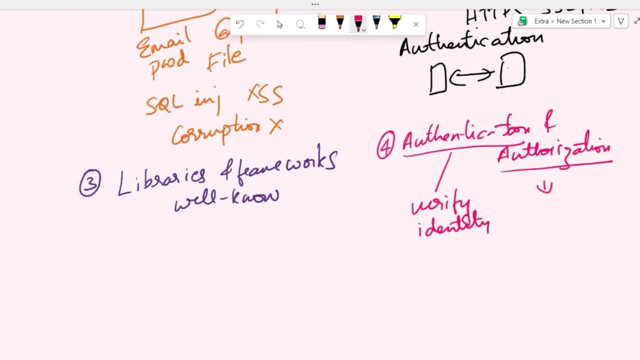 of a user and authorization tells us which user can do what. okay, so we need to implement secure authentication and authorization mechanisms to provide access to the users and make sure that they have appropriate access privileges based on their codes and permissions. then the fifth secure coding practice is related to the 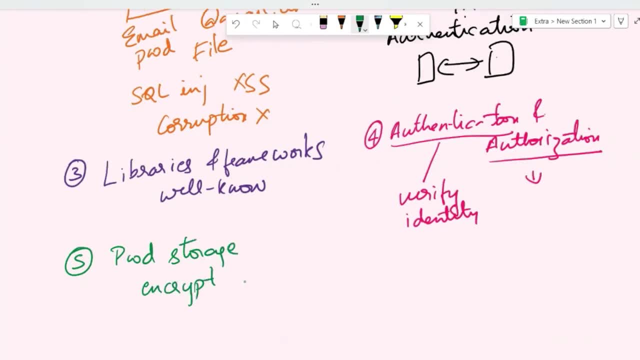 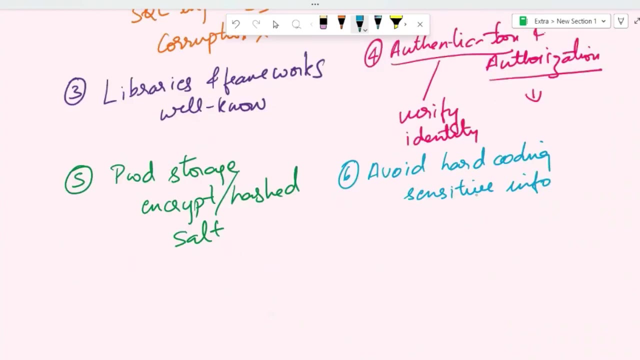 password storage. make sure that the passwords are either encrypted or hashed. you can also add salt to the passwords to prevent brute force attacks. okay, and passwords should never, ever be stored in plain texts. and another secure coding practice is to avoid hard coding sensitive information like, for example, your passwords. 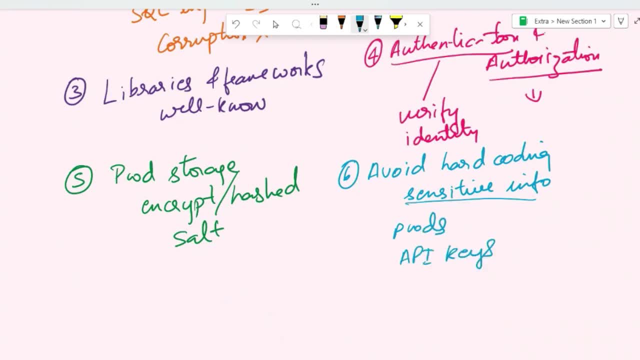 API keys or any other sensitive information in your source code. your configuration files or database tables right. never hard code them. like you can store sensitive information in environment variables which are separate from the source code and it might make it more difficult for the attackers to access it. proper error handling is required to prevent information leakage. 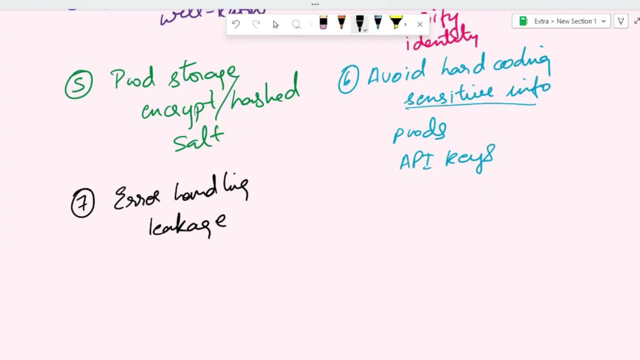 that can be exploited by any attacker. okay, like, for example, instead of showing a detailed error message, you can display a very generic error message, like, for example, in the show display page that we are talking, that is displayed to the user. okay, so you can all that you can have. 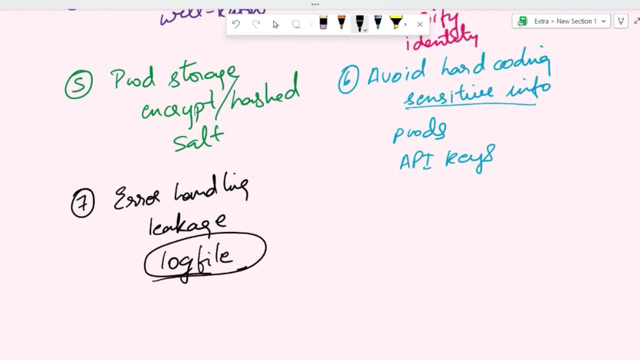 all the details in a log file and display very generic and minimal error message to a user like, for example, you can avoid revealing too much information about the server. like you know, stack traces or server software assertions should not be displayed. the next secure coding practice is to have the software updated regularly. 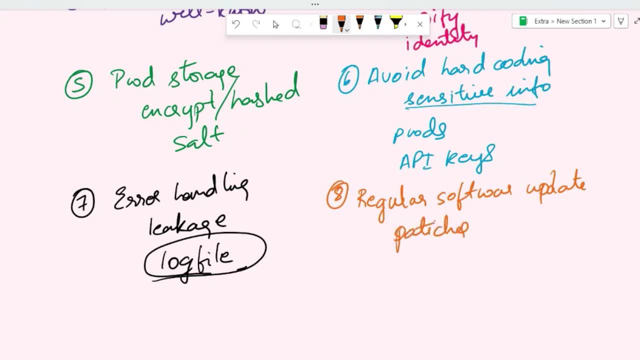 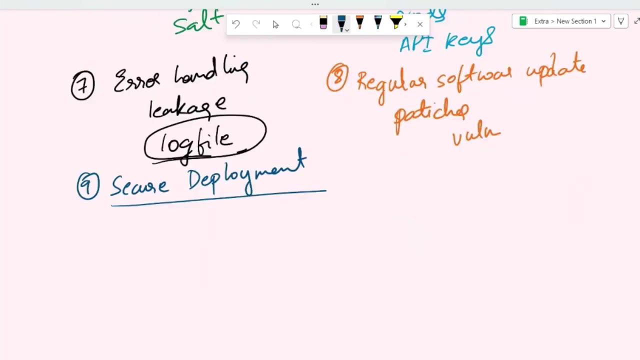 with latest security patches and fixes. This is to address any known vulnerabilities, okay, And you need to make sure that all software dependencies, frameworks, libraries, are all up to date with the latest security patches and updates. The next practice is secure deployment. 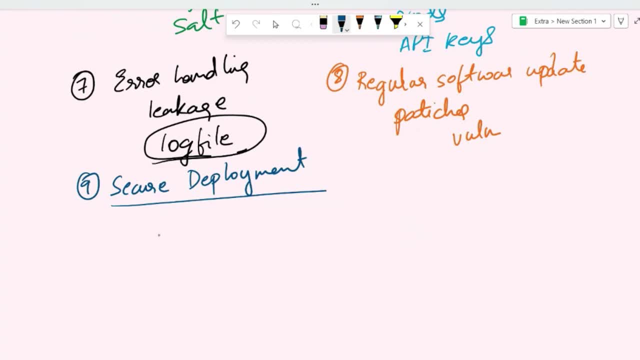 Make sure that you securely deploy the software by minimizing the attack surface. That is, you're using security configurations and secure infrastructure. Example: you can deploy the applications in secure containers and use secure network configurations to protect any unauthorized access. Another secure coding practice is awareness and training. 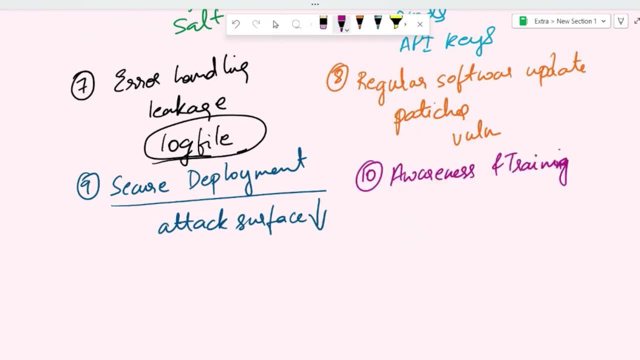 This is to provide security awareness and training to the developers so that they know what is a secure coding practice and how to mitigate risks. Why is it important And how does it affect an organization? The next coding practice is security testing. That means you are performing regular security testing. 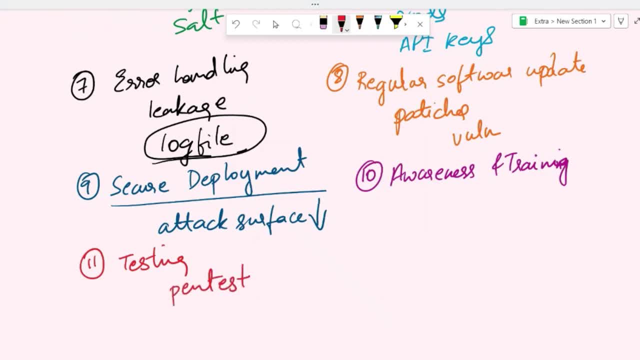 such as, you know, pen tests- That does, penetration testings- or code reviews to identify vulnerabilities and weaknesses in the application's code. This allows us to proactively address any potential security risks. okay, You can use automated security testing tools for this. 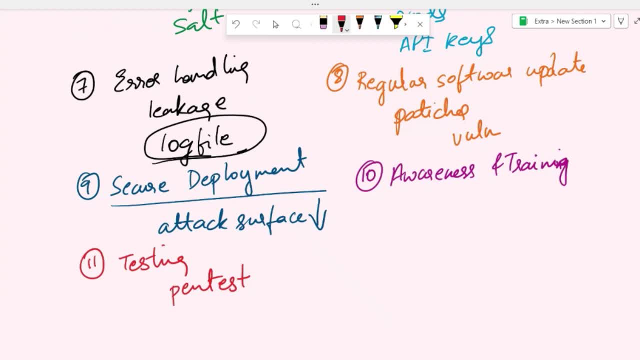 You can also hire a security expert to conduct penetration testing and identify any vulnerabilities. The next practice is secure third-party dependencies. That means in coding it refers to the external libraries or frameworks or components that the developers utilize in their software applications. okay, 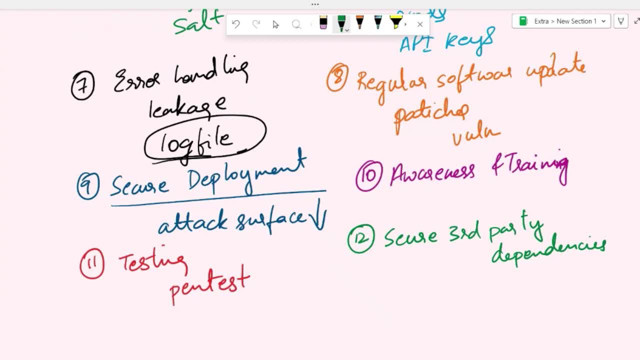 You have to make sure to use these dependencies in a very secure and responsible manner to minimize the risk of introducing vulnerabilities or any weaknesses into an application. Why do people usually use third-party dependencies? It is mostly because they're not used to it. It's mostly because to save time and effort. 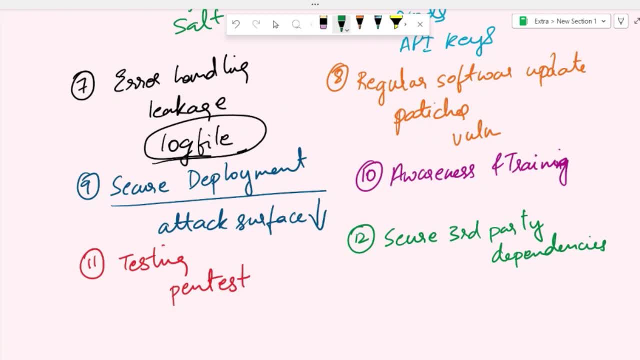 in creating their own, okay, But at the same time you have to make sure you evaluate the security of these dependencies and when they're kept up to date, you have to keep monitoring the security advisories. The developers should stay informed about any security vulnerabilities. 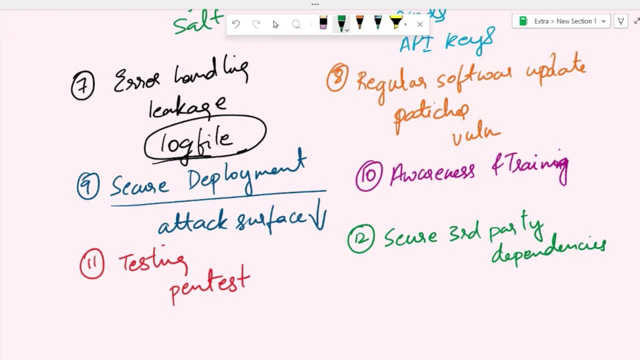 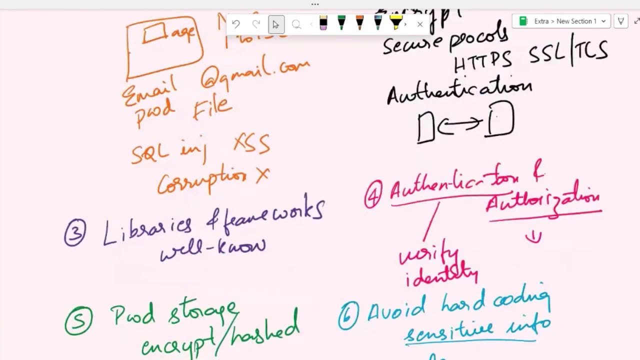 associated with their third-party dependencies, or if there is any patch released for these third-party dependencies that needs to be deployed. So these are some of the key secure coding practices, Something that I forgot to mention while talking about authentication and authorization. this also refers to access control.